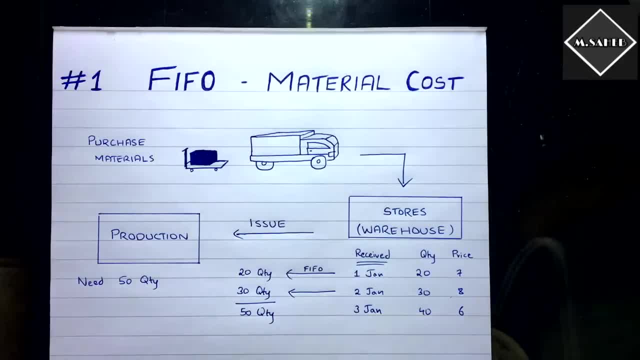 to the, to the showroom. yes, that's what happened normally in the business. so now here, what we do in FIFO method is: whatever that has come first into the warehouse in that order, only it will go out first. simple as that. that is what is FIFO: first in, first out. 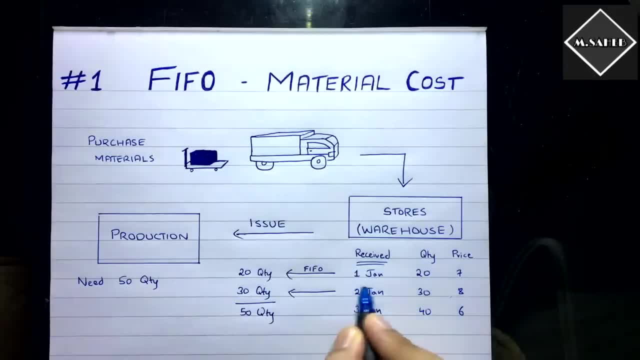 see, it's very simple. let's say, for example, on first January your warehouse received 20 quantity at the price seven. okay. and then on second January, let's say, it received 30 quantity at the price eight. and on third January it received 40 quantity of raw material at price six. right. so now let's say the production. 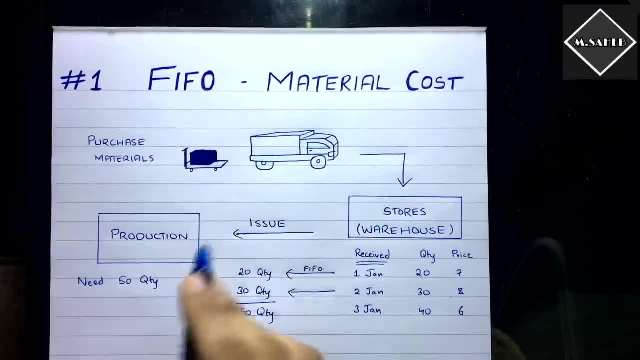 department requested that it is in need of 50 quantity and it made a request to the store department. okay, so now how the store department will release those 50 quantity. it will release in a particular order because they are following FIFO method. let's say, in this example they are: 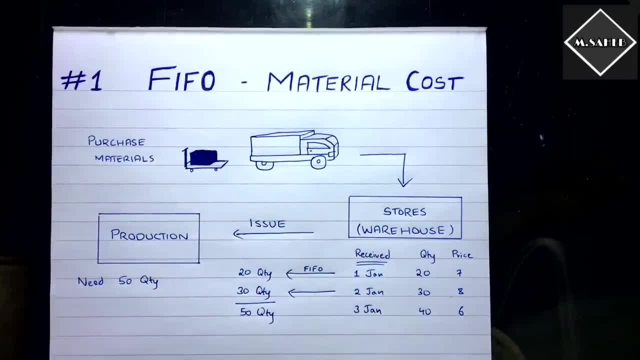 doing that. they are following FIFO method. so in FIFO method what happens? whatever comes in first, it has to go out first. so what came in first? 20 quantity at the price 7 came first on 4th January. so they need 50. yes, they need 50. so 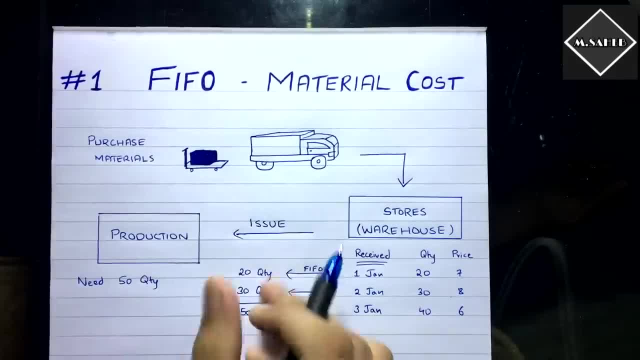 first you will pick this 20 at the price 7, 20 quantity at the price 7, and then you will pick, and then you need 30 more, right? so you will pick 30 at the price 8, right? so in this order, first in first out order, right, in this order, you will. 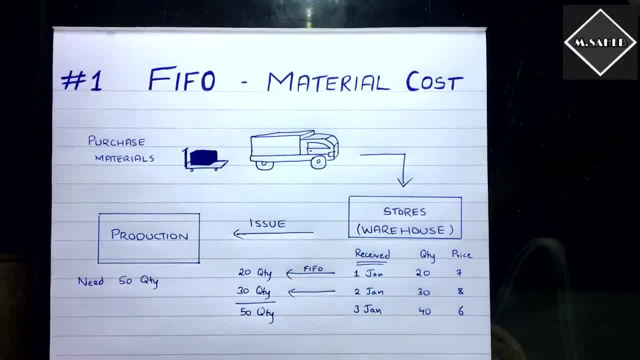 pick this and you will send it out to the production department. this is what is FIFO. so now you will be wondering how dervaluation is coming. you'll see, here we are not just taking the quantities in that order, the price also. so that is what the valuation is. that is how the inventory will be valued. first in first. 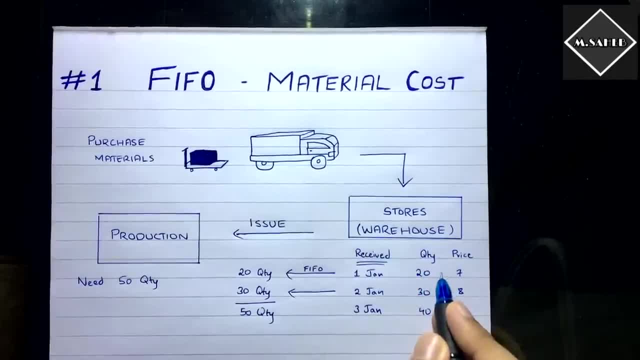 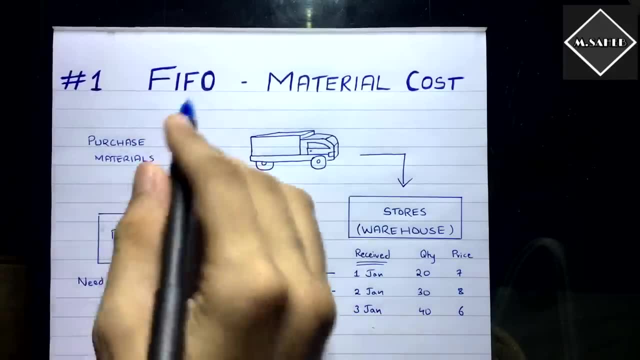 out whatever we purchased first from the supplier, in that order we are sending them out to the production department department. yeah, so that is how we are doing the valuation through the fifo method. okay, and then there is life. also, that is exactly opposite. we'll see that later in another video. yeah, so this is. 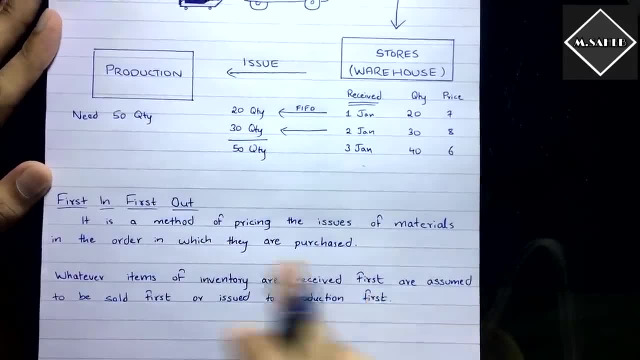 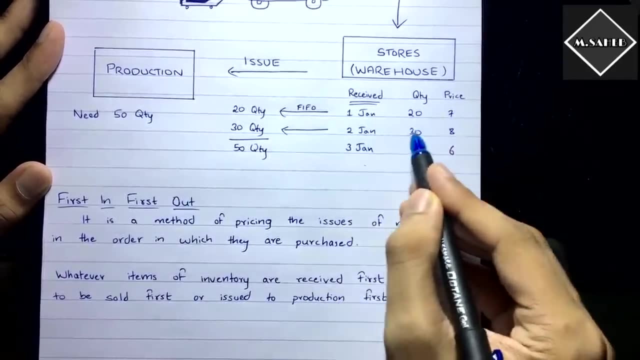 what is fifo method? it is a method of pricing the issue of materials in the order in which they are purchased. right, you purchase them, see here: on 1st january you purchase 20 quantity. on 2nd january you purchase 30. on 3rd january you purchase 40, and at these prices. so now how they will be released. 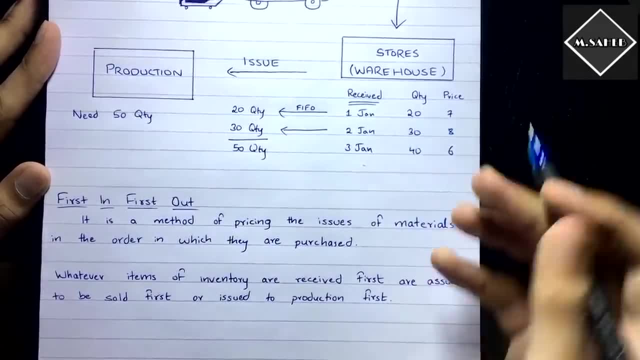 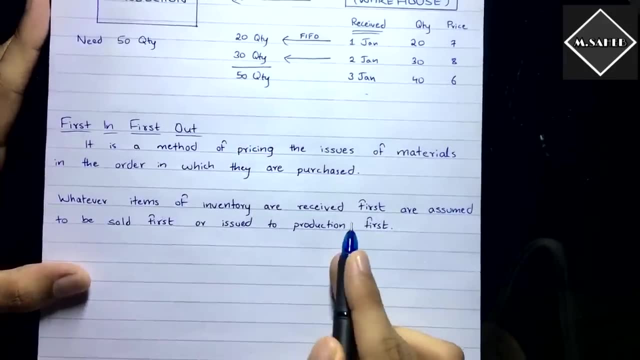 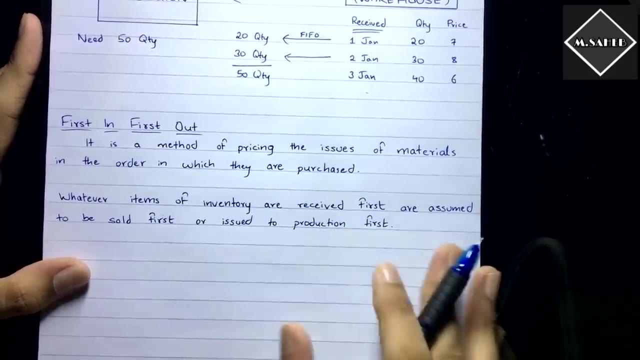 to the production department in the order they were purchased. okay, you see this, this is what is first in, first out. method of inventory valuation. yeah, whatever items of inventory are received first are assumed to be sold first or issued to the production department first. okay, this is what. 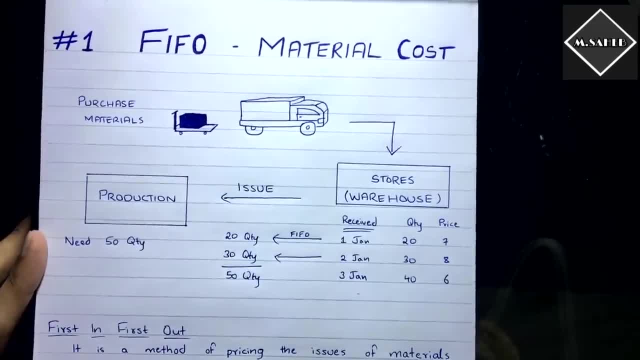 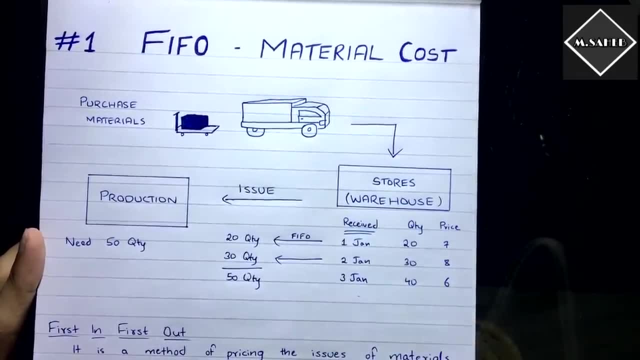 is fifo method. now let's solve a problem on this and you will understand what is this fifo method? okay, whatever comes in first, it has to go out first. it's very simple, right? and the life is exactly opposite to that. we will see that in another video. 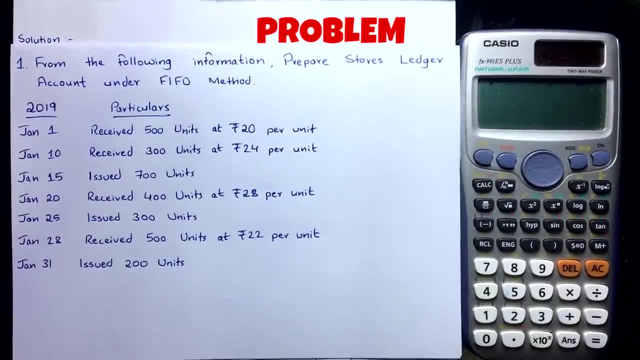 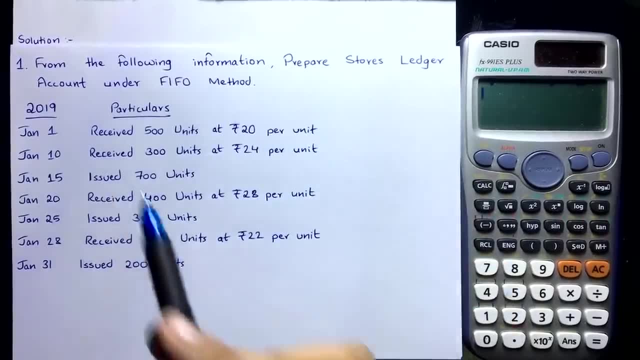 now let's go to the problem of fifo. now, here we have the problem. see here from the following information: prepare stores ledger account under fifo method. right, so now? what is this store ledger? store ledger is an account that is prepared by the warehouse to keep the track of materials. 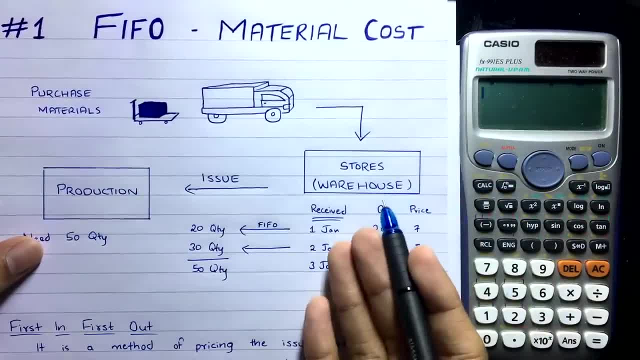 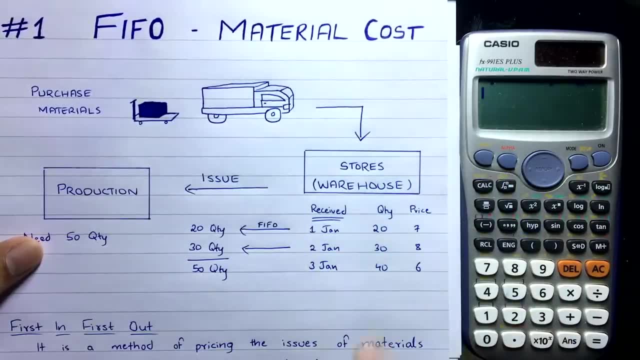 how much material has come into the warehouse and how much material has gone out of the warehouse and how much material do they have right now in the warehouse. okay, to keep track of the materials, that stores ledger account is prepared and in all the process of preparing the store ledger account, 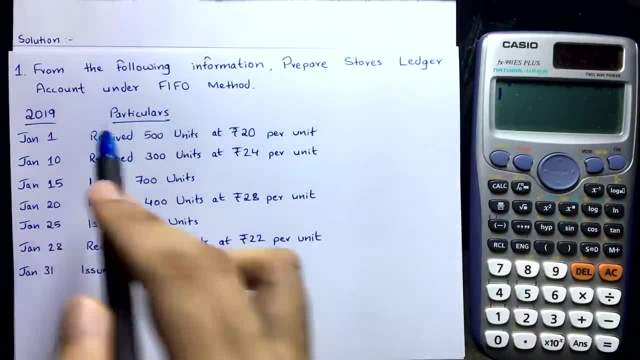 what are the problems? what are we going to do? we are going to prepare that store ledger only. okay, it is prepared under different, different methods. okay, now here we are discussing about fifo method. so we are preparing stores ledger under fifo method, first in, first out method. see the question here. 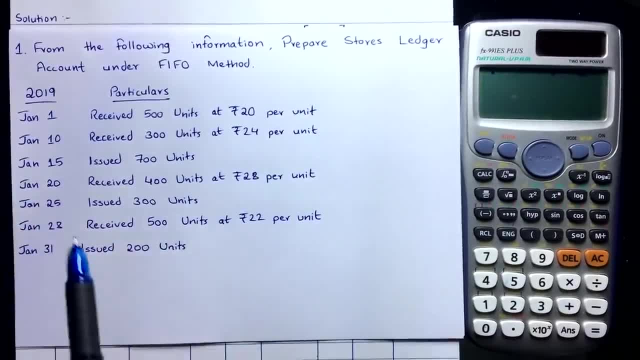 it's very simple now. first, they have said: on january 1st 2019, we have got 500 units from our supplier. right, we have received 500 units at rupees 20 per unit. now here you have to think from the point of view of the warehouse: okay, what has come into the warehouse? what has gone out of the 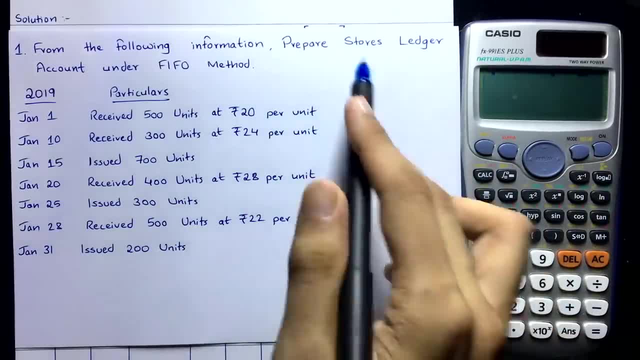 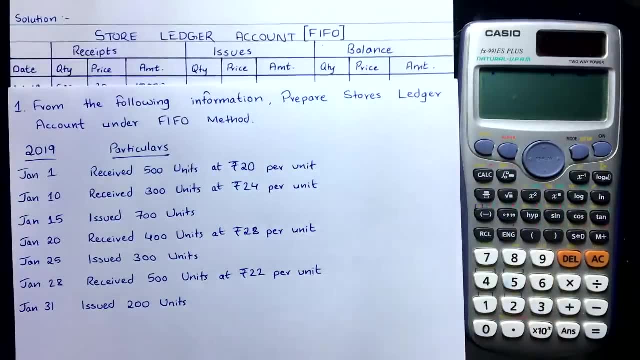 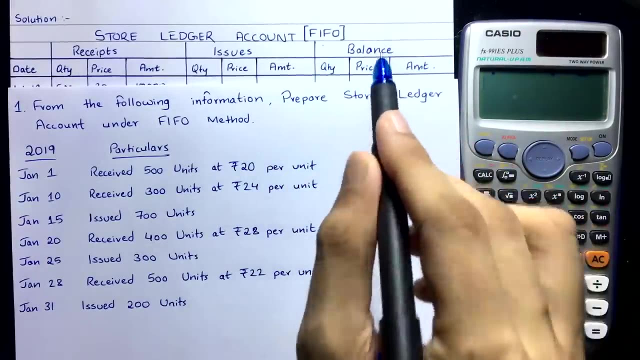 warehouse understood. yes, so first you have to understand the format of stores ledger. see, the format is very simple. you have got date column, receipt column, issues column and balance column. yeah, receipts means what has come, issues mean what has gone out and then balance mean whatever that is there in the warehouse right. and then in these three columns- receipts, issues and balance- 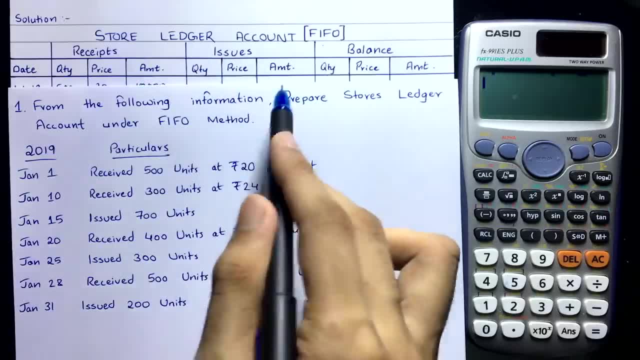 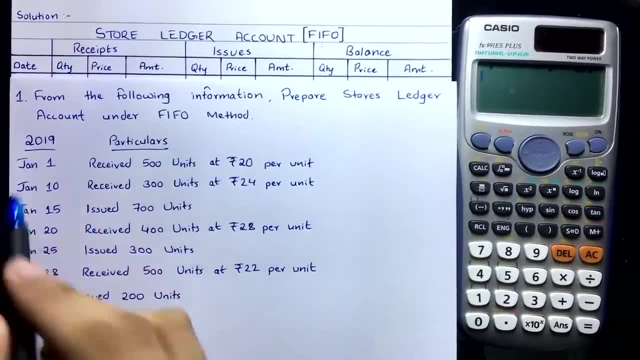 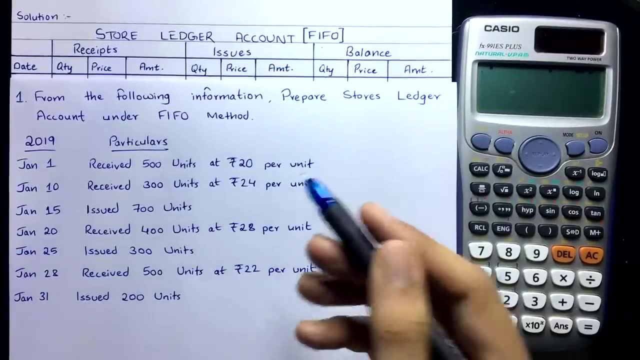 there are three more sub columns: quantity price amount. quantity price amount. quantity price amount. fine, okay, now the first action that we have got is see here: on first january 2019, we have received 500 units in our warehouse. add rupees 20 per unit. simple, it is a receipt. yeah, we have got that in our warehouse. 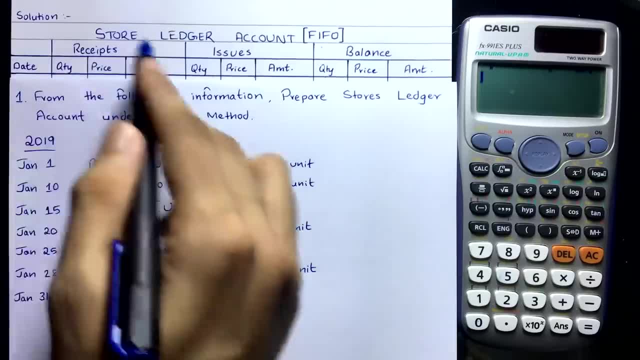 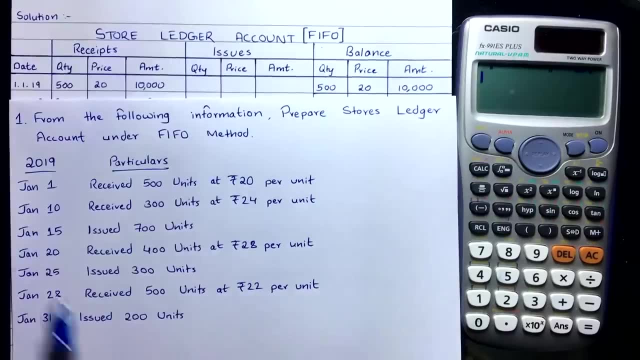 we have to see from the point of view of warehouse. so it will come on the receipt side. we have got the quantity and price and if we multiply that we will get the cost, the amount, simple. just copy that down. on first january 2019 we have got 500 quantity, add the price, rupees 20 into 20. that is. 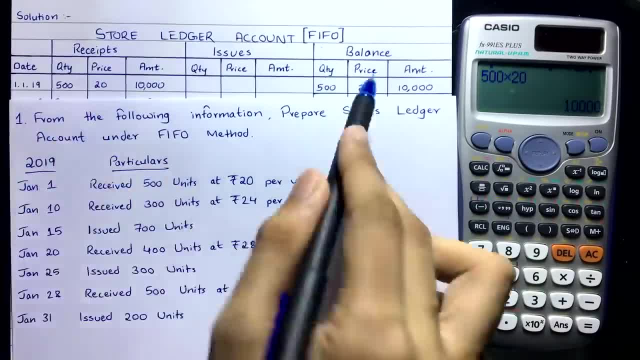 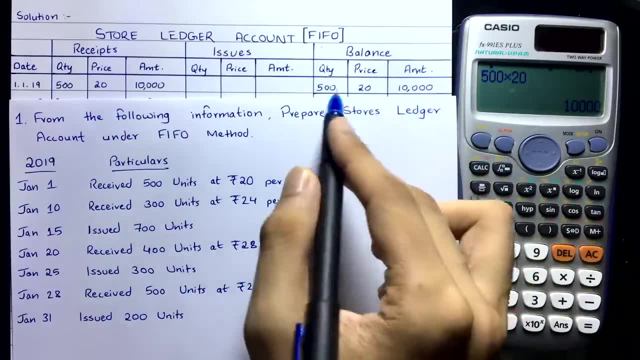 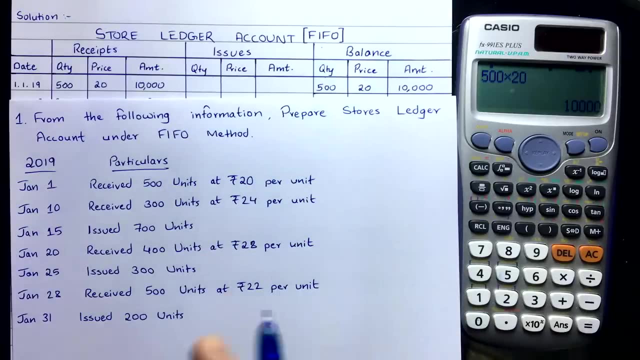 the total amount, then what you have to do? you have to copy that down to the balance column. yeah, balance mean what balance means? you have 500 quantity right now in our warehouse. yeah, so 520, 10 000.. simple, you have to copy that exactly down. yeah, or if there is an opening stock, that is given. 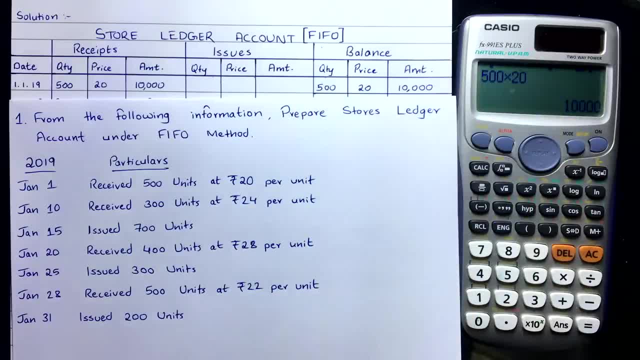 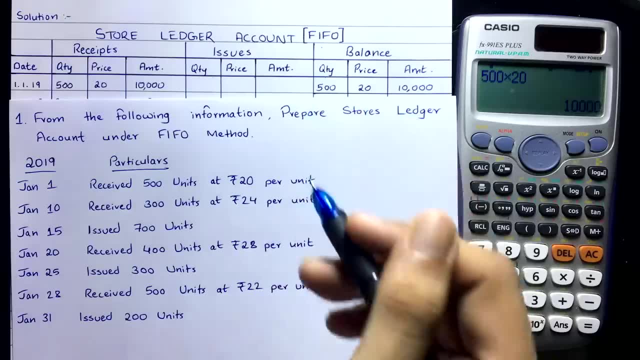 to you in the question, then you have to directly take that into the balance column. yeah, you didn't receive that right now. it's just a balance. yeah, whatever that was there from previously. if opening stock is given in your question, yeah, but here you have to copy that down to the balance column. yeah, 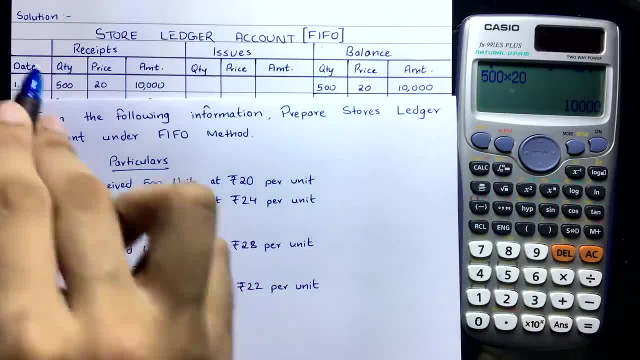 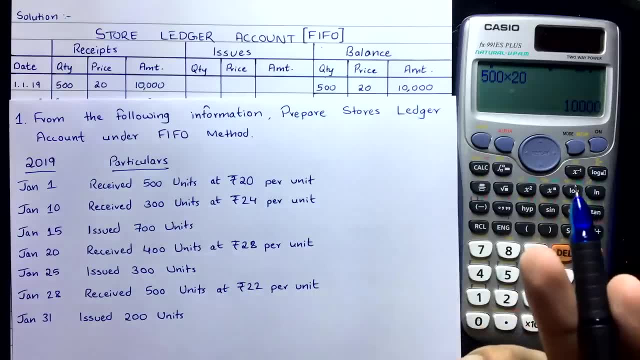 here. they have said we have purchased, we have received 500 units. so first you have to take into the receipt column and then copy that down exactly in the balance column. yeah, the first receipt will always be like this: okay, fine, and then what you have to do, and then you have to go. 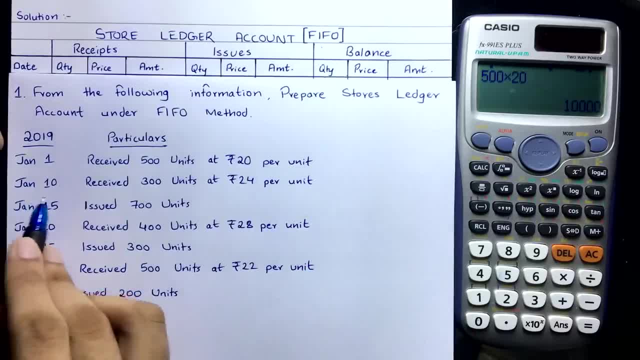 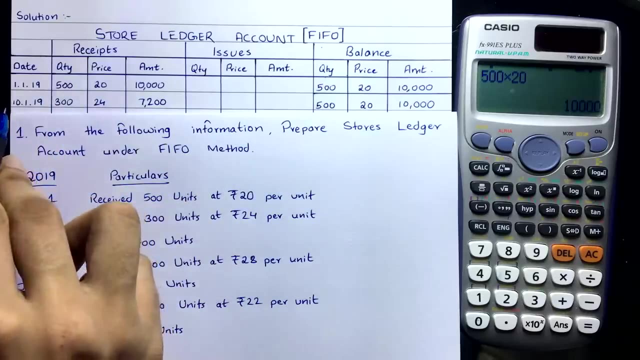 to the second transaction on january 10. yeah, 10 january. what has happened? we have got another receipt. see here we have received 300 units at rupees 24 per unit. fine, it's very simple. so what you have to do, you have to write that down in the receipt column. on 10 january, we have got 300. 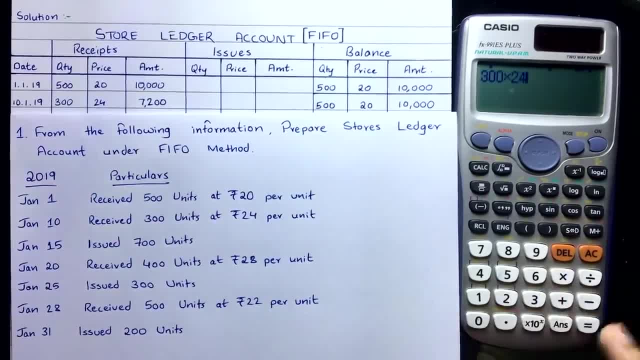 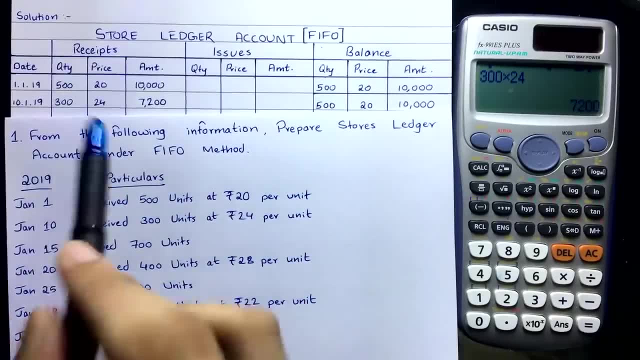 quantity: add the price: 24, 300 into 24, that is equal to 7200. yeah, yes, simple yes. now how will you copy this, the second receipt, into the balance column? how will you do that? that is the main thing. okay, most of the students, they make mistakes over there. if you make a small mistake, right then your. 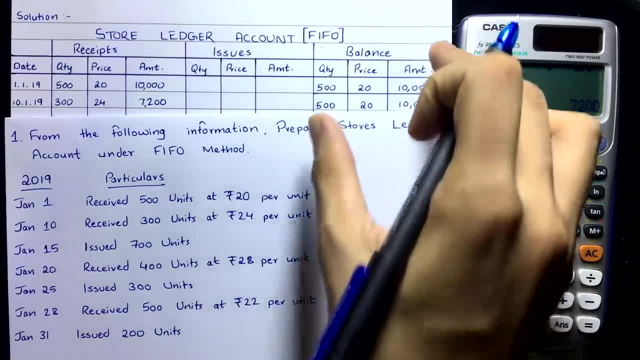 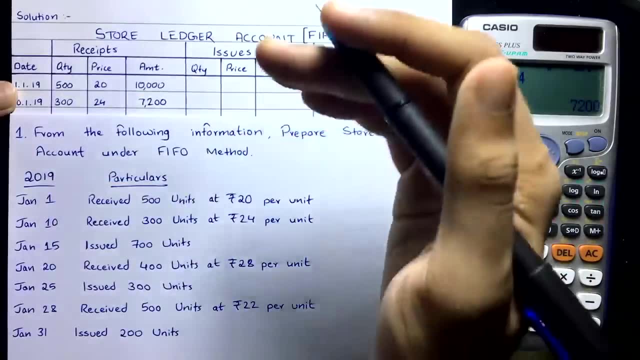 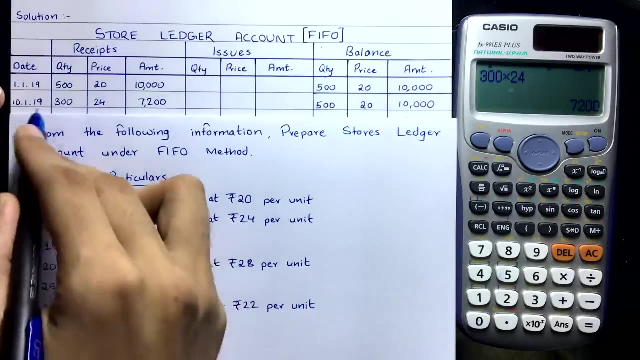 entire fifo problem will be wrong. so that is why the balance column should be done proper, carefully, okay. so see, it's very simple. whenever you get a receipt right, let's say: you are doing the fifo calculation, this statement, yeah, this account. then immediately let's say: you get a receipt, yeah. so whenever you get a receipt, what you have to do is 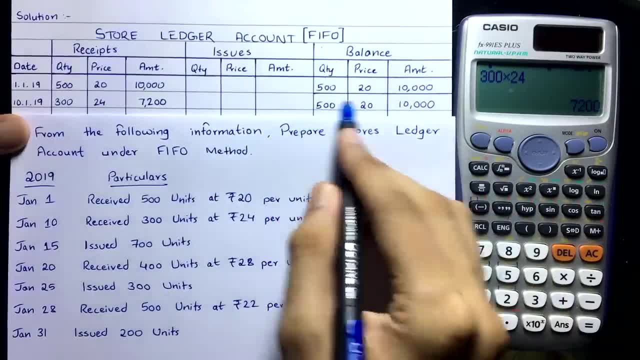 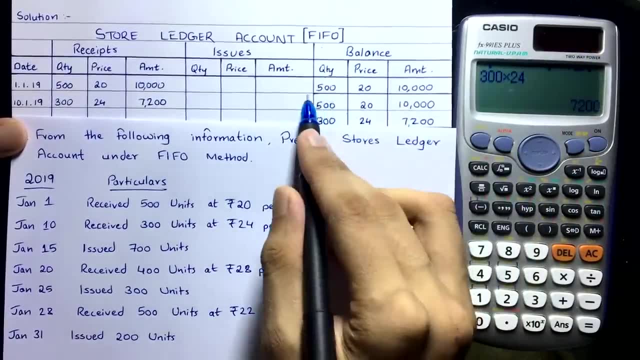 you have to draw a line in the balance column. okay, you have to draw a line, and then, whatever that was there in the balance column, you have to copy that exactly down. okay, see here, i drew a line over here, whatever that was there in the balance column. 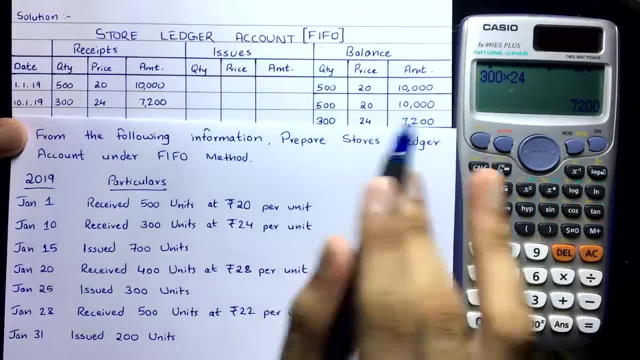 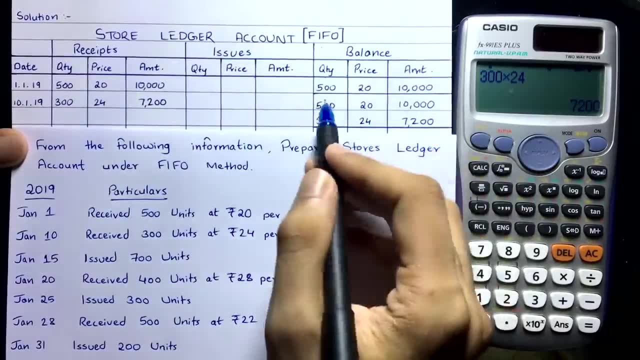 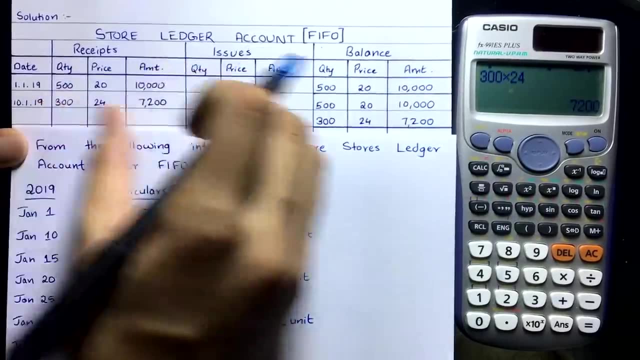 i took it below 520 10 000. exactly same, yeah, 520 10 000, yes, and then whatever received you have got, take that exactly below what you have copied just now. yeah, first take this down after drawing the line and then take this thing below that. okay, this is what you have to follow. 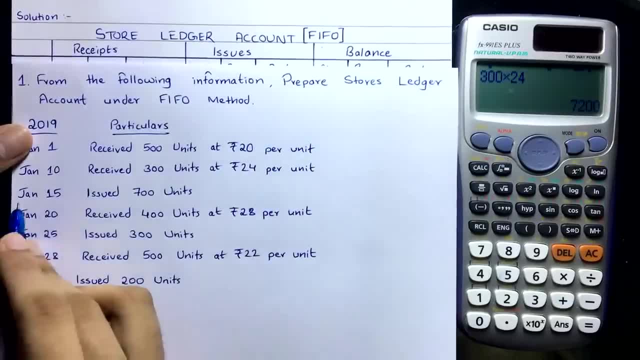 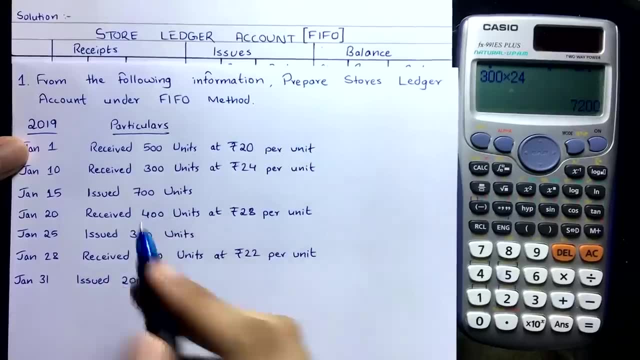 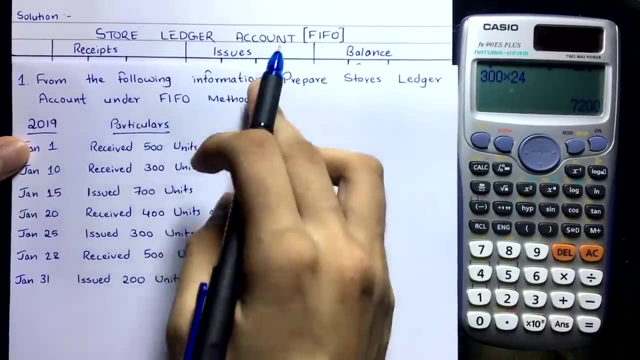 simple. let's move on. you will understand that on january 15, what has happened? we have issued 700 units. we have sent out units, probably to the production department. yeah, so how will you record this? this is going out of the warehouse, that is issues, so you will have to take that into issue. column simple: see here. 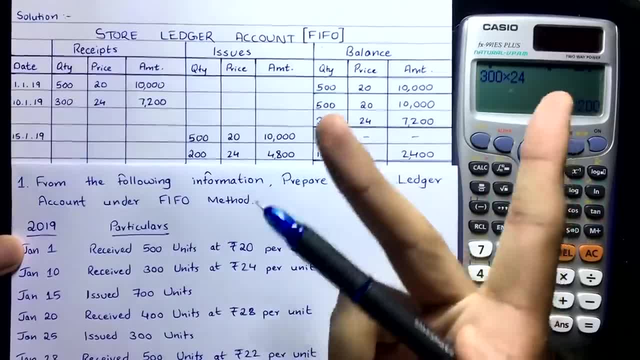 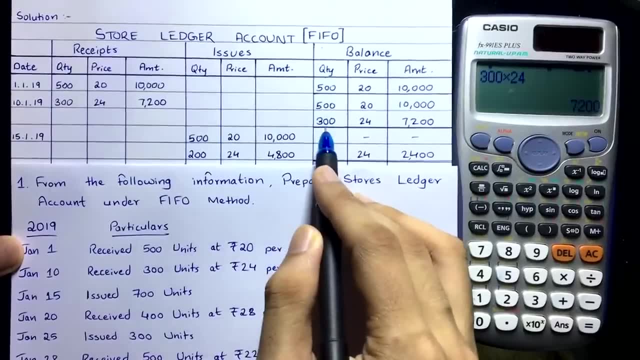 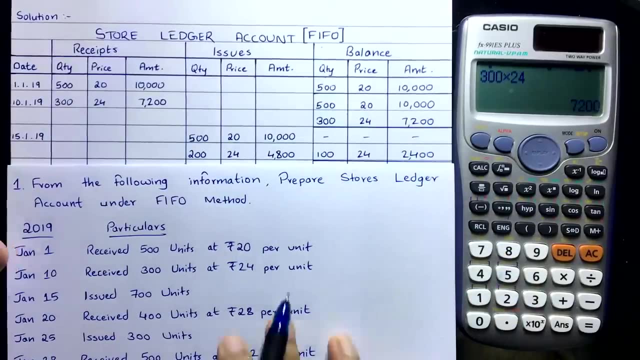 now, what do you have in the warehouse? in the warehouse you have two lots. one is 500, quantity lot of rupees 20 and the cost is 10 000. and another lot of 300. yeah, this lot, that was price 24, yeah, and the cost is 7200. so now you have to send out 700. yeah, as said in the question, 700. 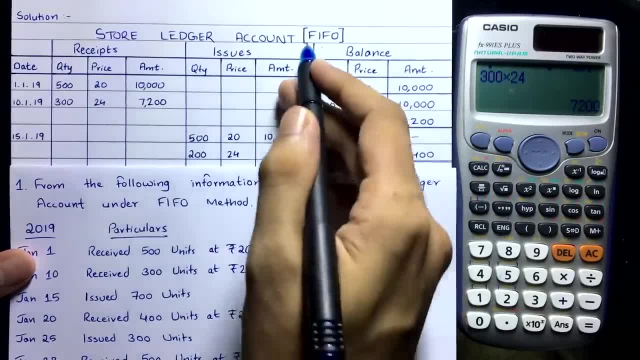 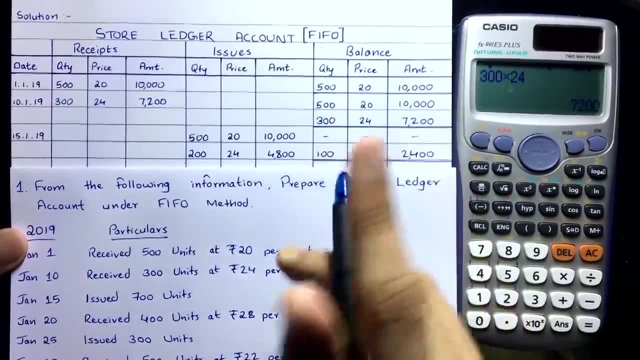 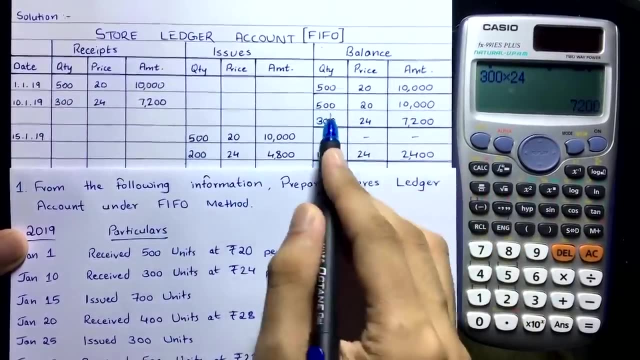 units. so how will you do that? you have to follow first in, first out. yeah, fifo method. how will you do that? first you will take out 500 quantity at this 20. yeah, you have to send out 700, yes, but first you have to take this first lot. yeah, first in first out. so first lot completely. and 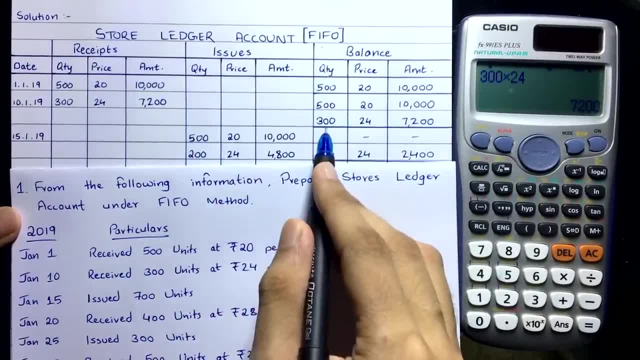 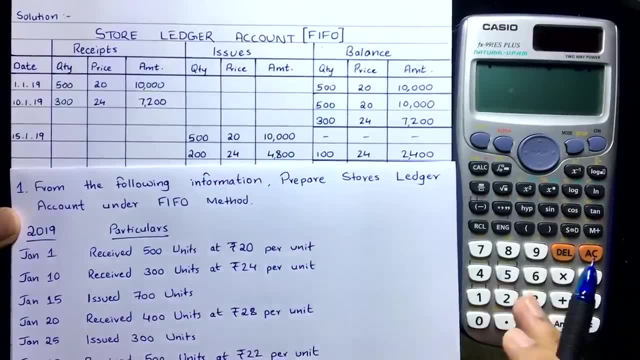 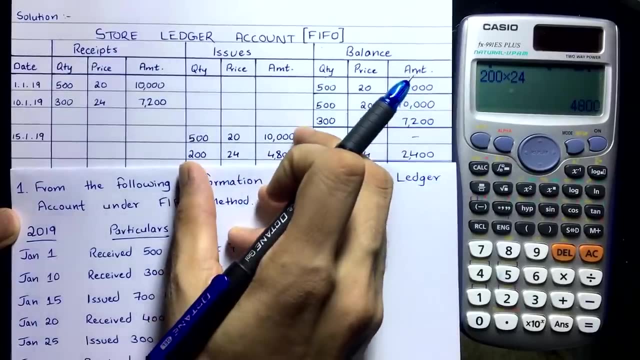 then you need additional 200. that will come from the second lot, from this 300 lot. okay, so 200 at the price 24. so see here, that's the same 200, then the second one. see here: 200 into 24, that is equal to 4800. yeah, simple. so this is what will go out of the warehouse. 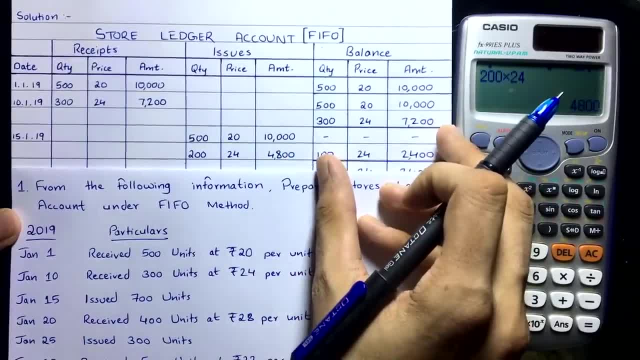 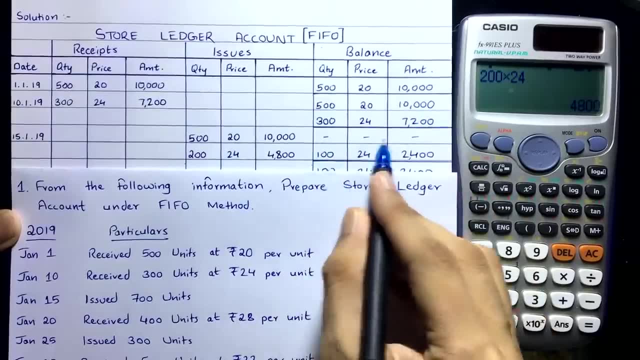 and then what will remain in the warehouse? what is the balance? how will you take the balance? now? you have to draw a line, okay, and now this 500 is no more. it has gone out of the warehouse. so nil, nil, nil, but here in the second lot. what has happened in the second lot in? 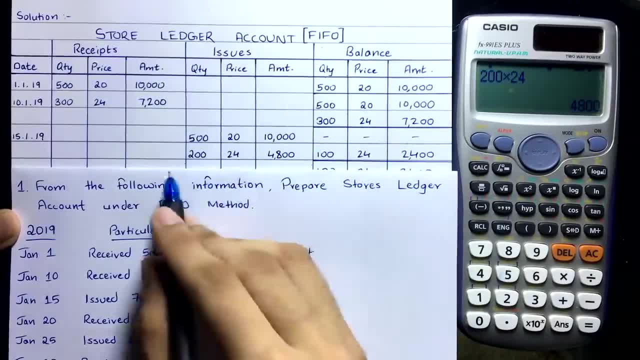 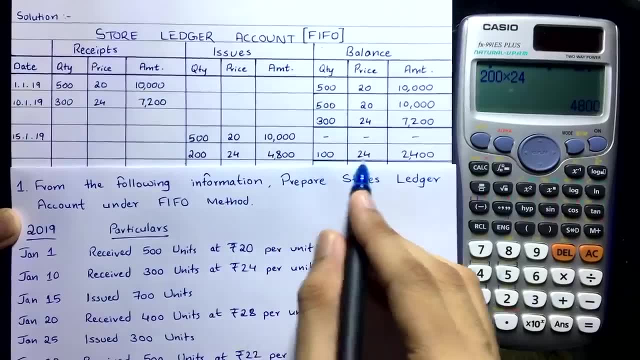 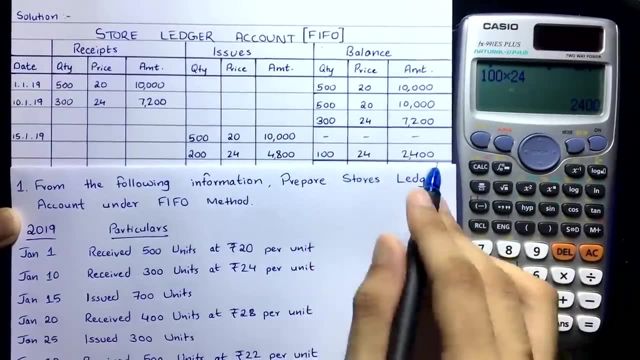 this 300 quantity, only 200 has gone out. so remaining, you have to take it: 100 is remaining. if 200 has gone out out of 300, 100 is remaining. yes, at price will be same: 24. so 100 into 24 that is equal to 2400. so 2400 is the balance that is left in the warehouse till here, you understood. 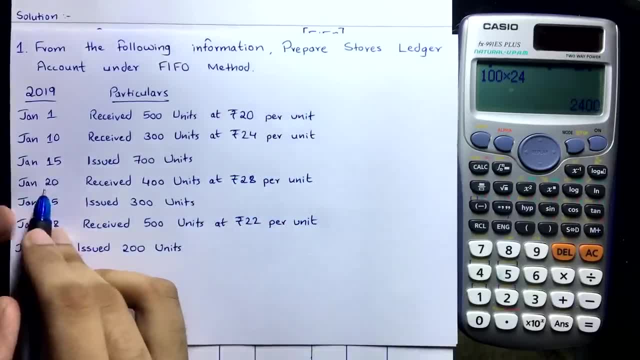 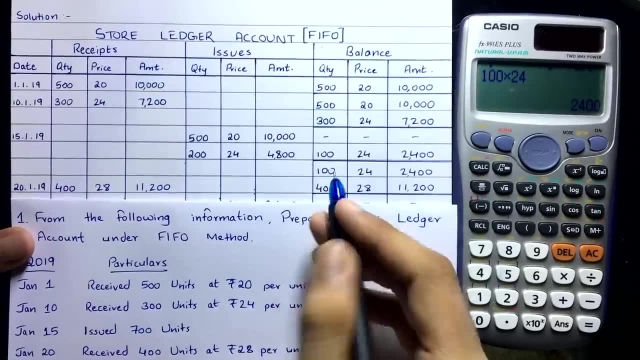 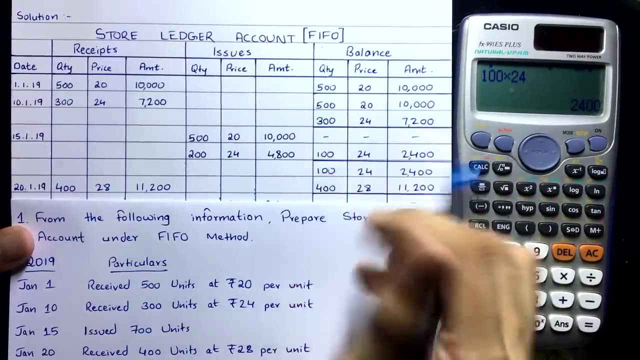 it's very simple. and then what happened? see here, on january 20 you got a receipt. now what i told you: whenever you get a receipt, go to the balance column. yeah, go to the balance column. draw a line. yeah, draw a line. copy exactly whatever that is there in the balance column 124: 2400 is there in. 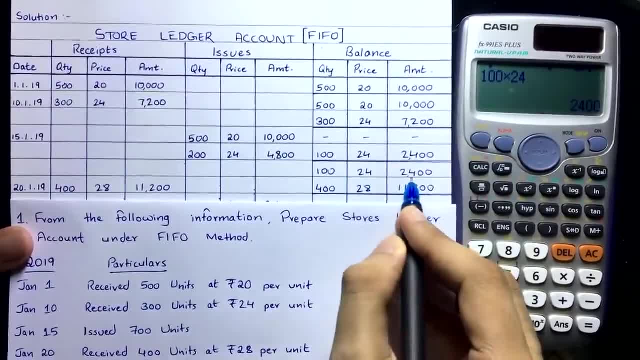 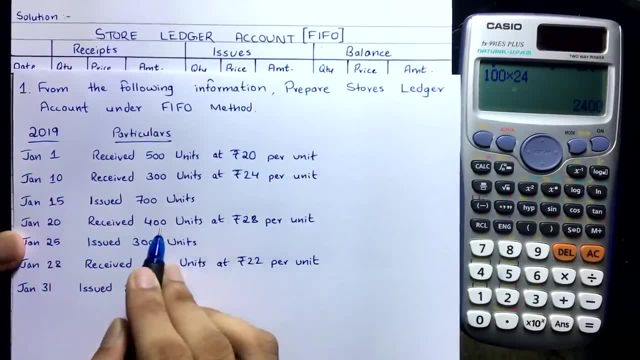 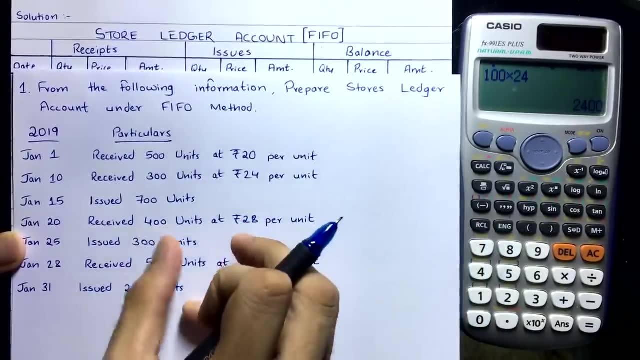 the balance column. copy that exactly down: 124, 2400. okay, and then go back to that transaction. on january 20 received 400 units at rupees 28 per unit. yeah, you have received in your goal down. you have received in your warehouse 400 units at rupees 28. copy that in the receipt column. 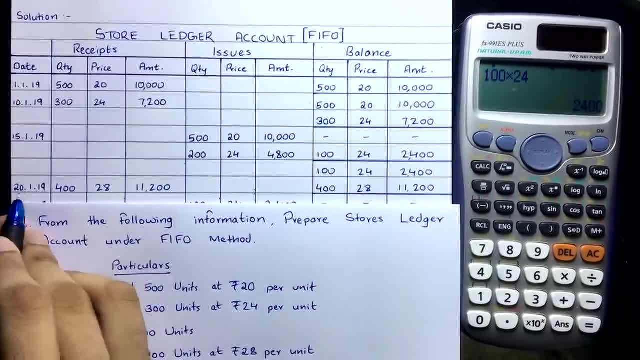 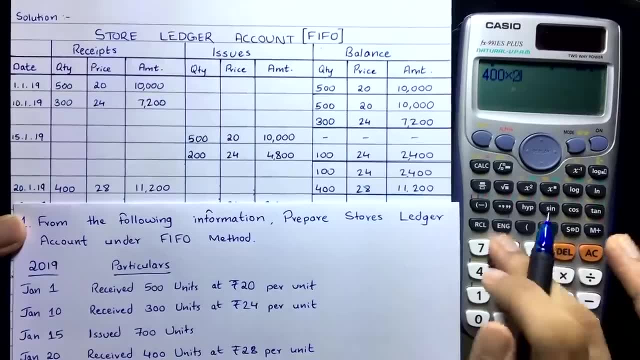 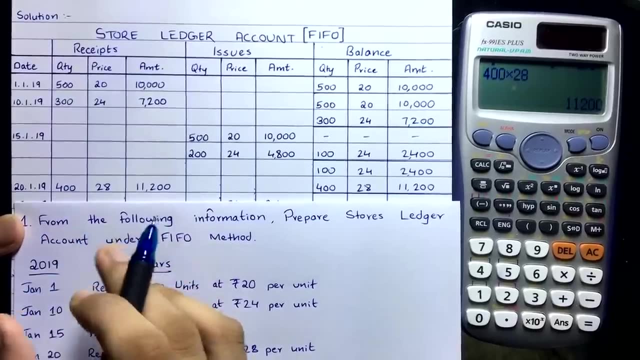 record that on january 20, yeah, on january 20, you have got 400 quantity rupees, 28, yeah, and the amount is 400 into 28. that is equal to how much 11 200? that is the cost of 400 quantity, right, but what i? 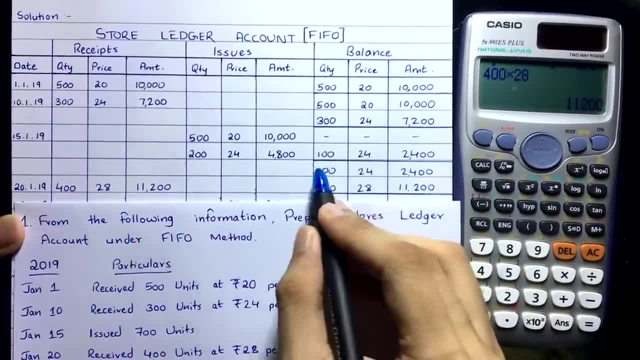 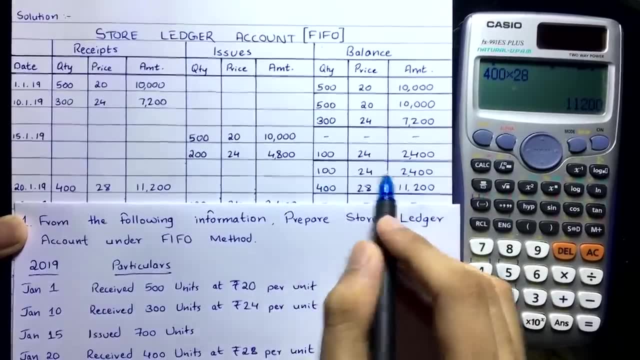 told you, whenever you get a receipt, what you have to do: draw a line in the balance column, copy what that is there previously in the balance column down. yeah, you did that. and then you have to take this receipt. exactly below that, you have to take this. you have to copy this and paste it over here. 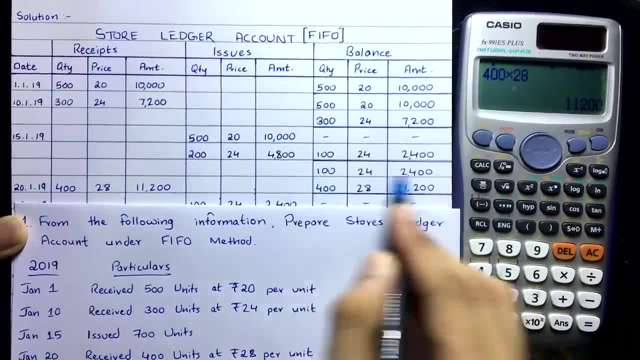 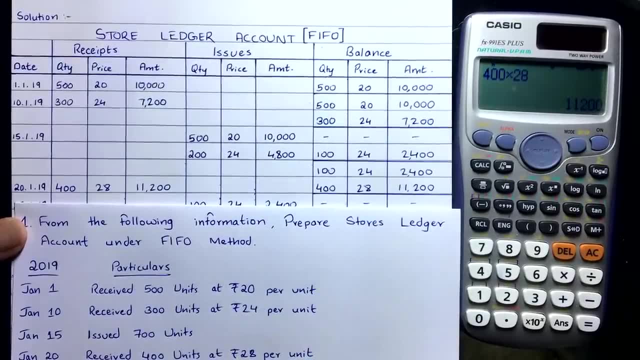 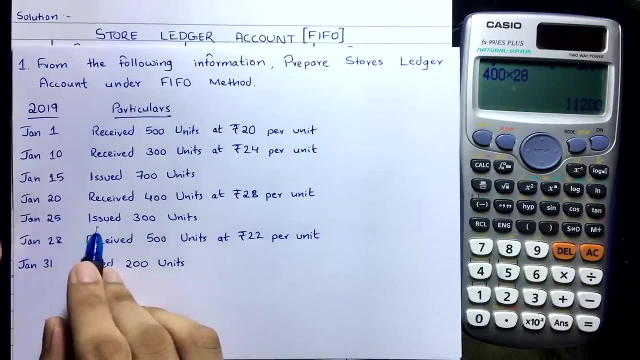 right, you understood. copy this down, yeah, whatever that is there in the balance column, and then take this below that simple yes, and then move on. you're getting it right what i'm telling you. yeah, and then move on. see here. and then, on january 25, what happened on january 25: issued 300 units at rupees 28. 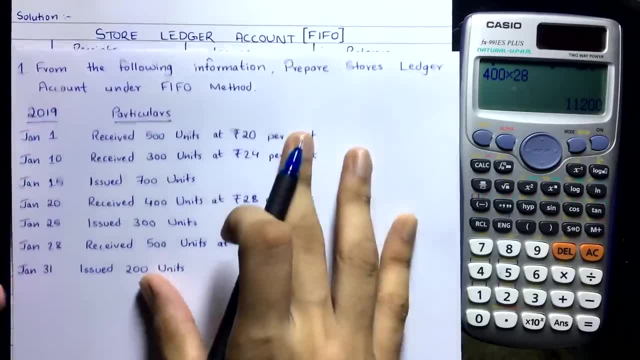 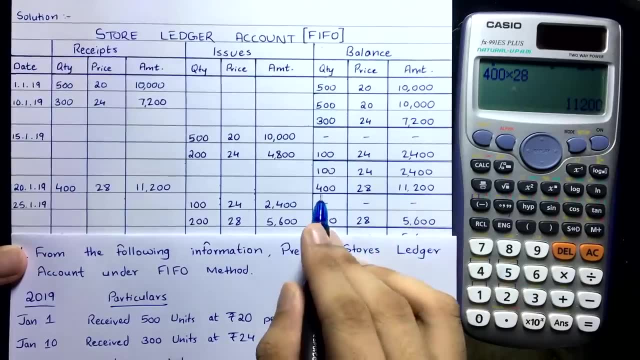 units, we have to send out 300 units. yeah, we are following fifo method. so see, here we have two lots now. one is 124- 2400, and then the new lot which we got right, that is 428, 11, 200. yeah, so what you have. 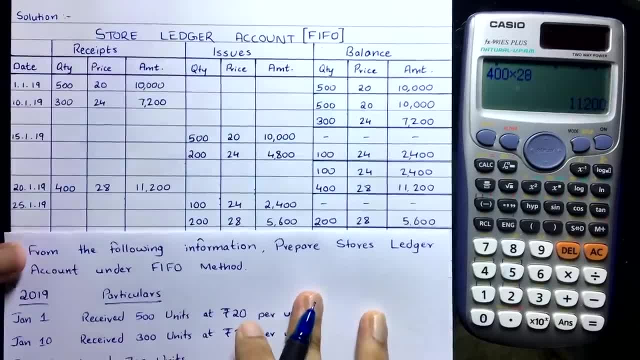 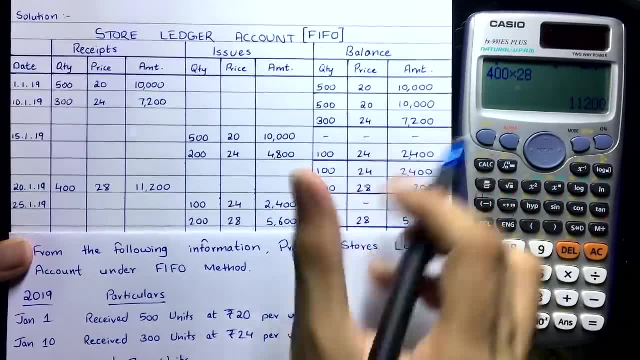 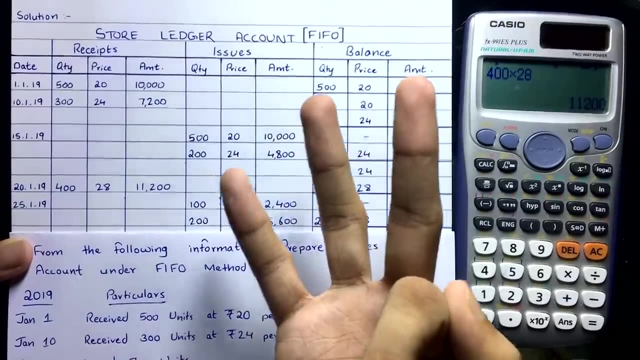 to do is you have to send out 300 units. so how will you do that? simple, first in, first out. whatever that is first, you have to send that out first. so 100 is first. so you will send out 100, 124, 2400, yeah, and then the remaining 200. you have to send out 300, right, as said in the question, but you have 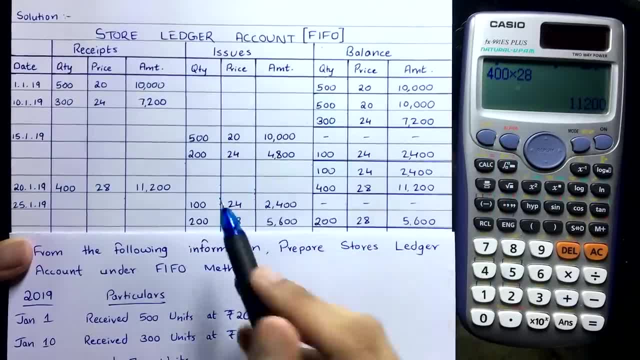 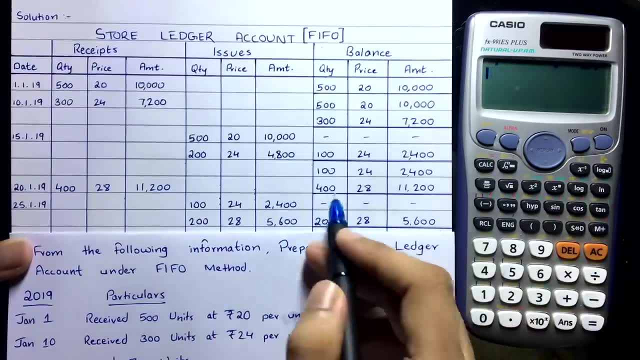 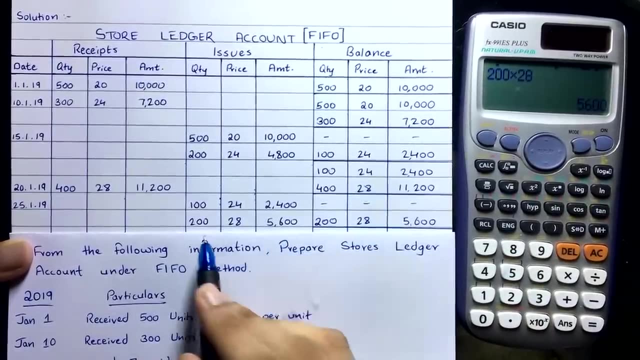 sent out only 100, so additional 200 has to be sent out so that 200 will come from the second lot. okay, 228, okay, see here: 228. the price is 28, so 200 into 28, that is equal to 5600, simple 200. 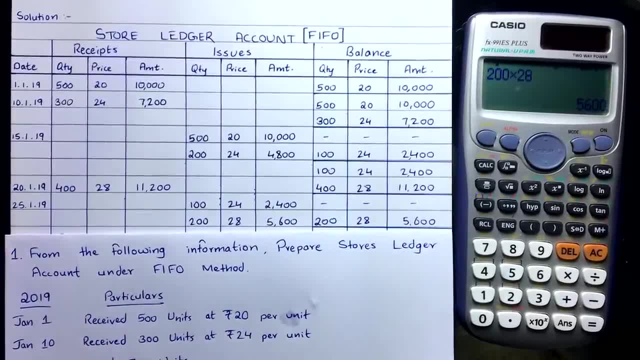 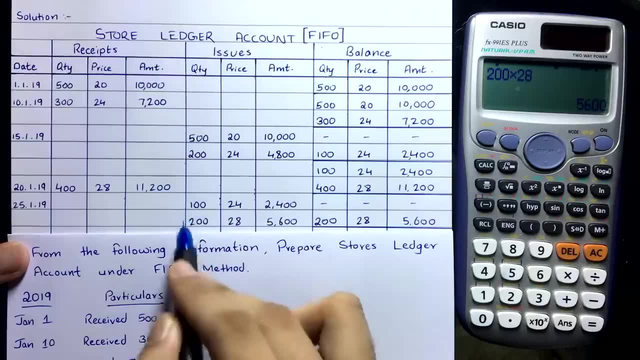 into 28, that is equal to 5600. now you have to send out 300 units, right? so you have to send out 300 units, right? so you have to write the balance. how much is left in the warehouse now after sending out these 300 quantity? see, here, it's very simple. this 100 is entirely gone. nil, nil, nil, yeah. 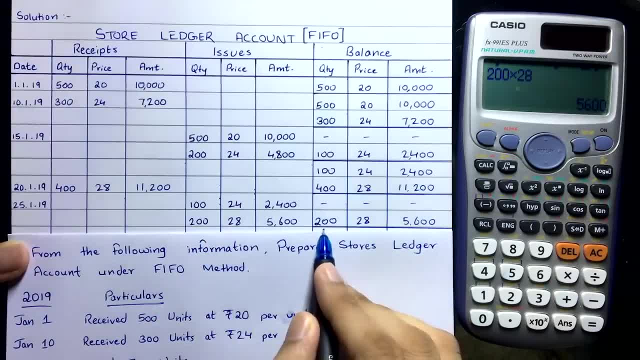 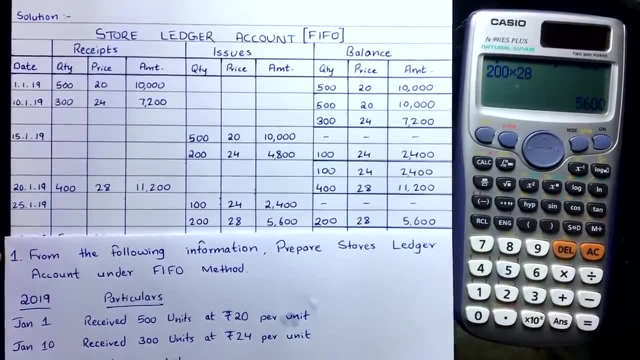 now, from 400, you have sent out 200, so the remaining is 200 and the price is 28, so 200 into 28, that is equal to 5600, simple. yeah, so this is what is left in the warehouse. how much quantity? 200 quantity. 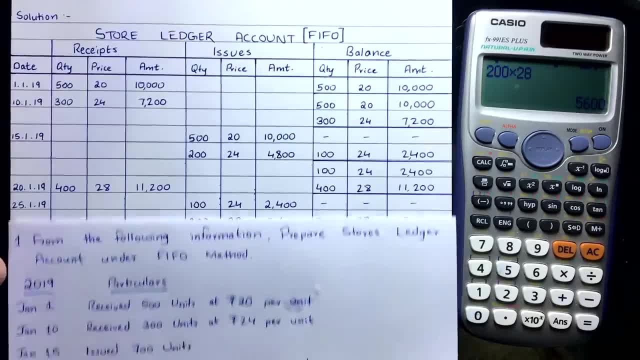 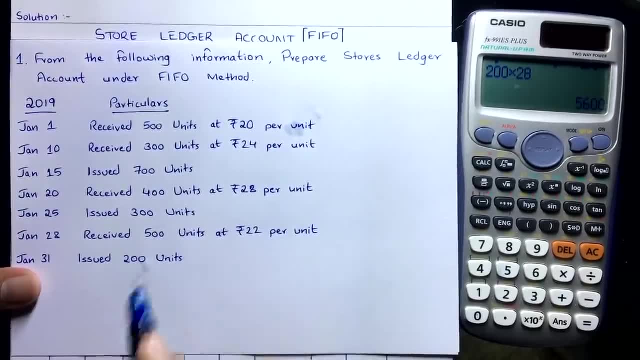 of rupees 28, the cost is 5600. and then what happened? move on. on january 28, you have got another receipt of 500 units. what i told you: whenever you get a receipt, draw a line in the balance column. see here: draw a line in the balance. 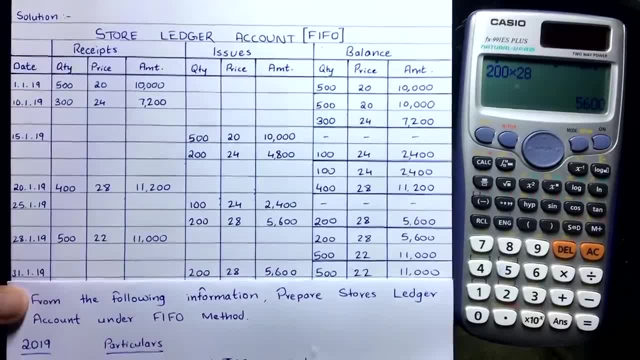 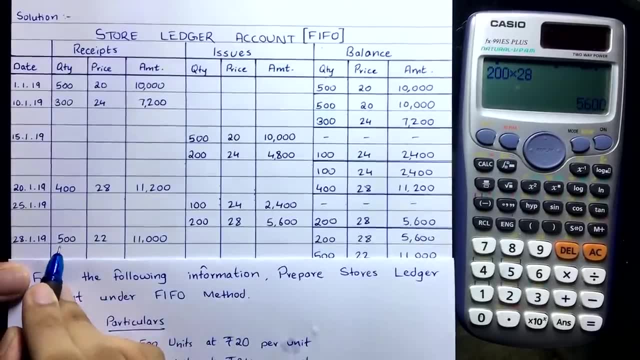 column and then copy the receipt. first see here what has happened. we have got 500 units, add rupees 22, right? so you? we have got 500 quantity, add price 22. so 500 into 22 that is equal to 11 000. yeah. 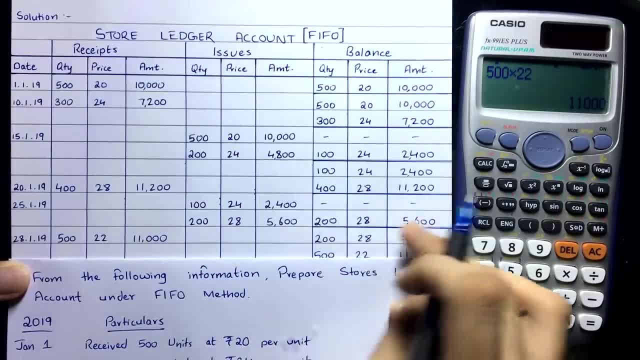 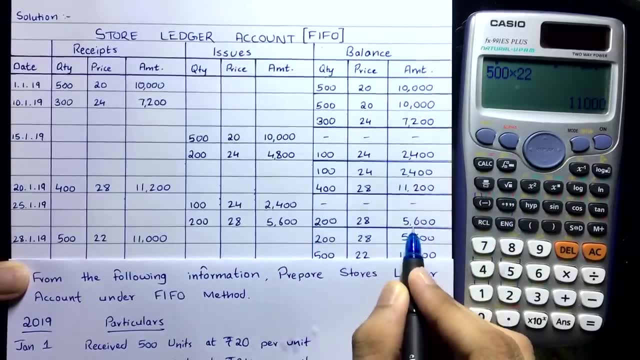 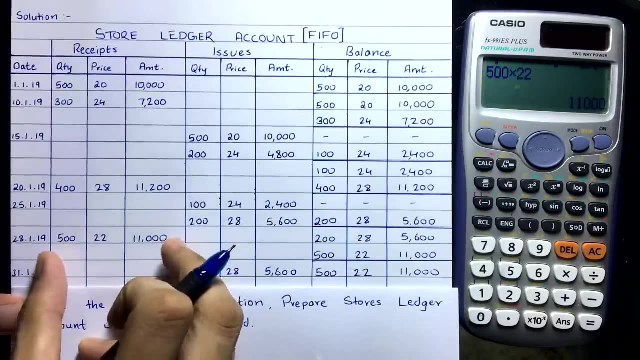 11 000. and then what do you have to do? in the balance column, draw a line, copy whatever that is there in the balance column previously. copy that down exactly 228 5600. copy that exactly down 228 5600. yeah, and then what you have to do is whatever that you have received now take that. 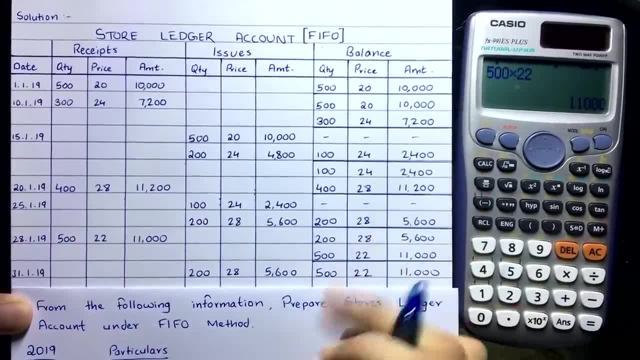 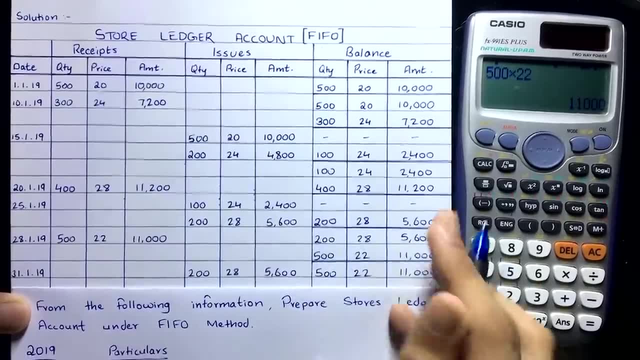 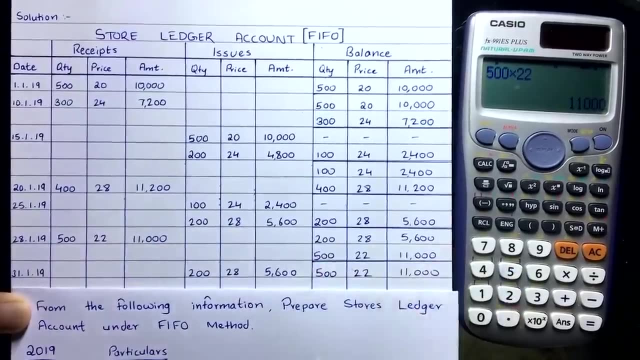 yeah, copy it and paste it exactly below that. 520 to 11 000, simple. yeah, this is what we do whenever we get a receipt: draw a line, whatever that is there previously in the balance column, copy that down and whatever you have got just now, copy that below. understood, yeah, and then the last transaction. 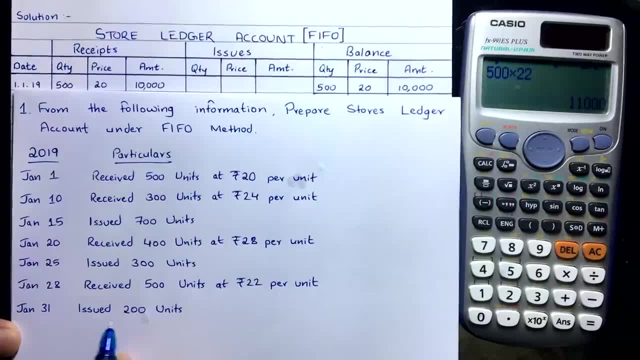 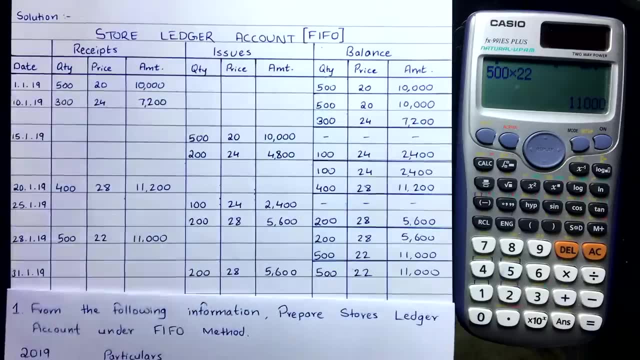 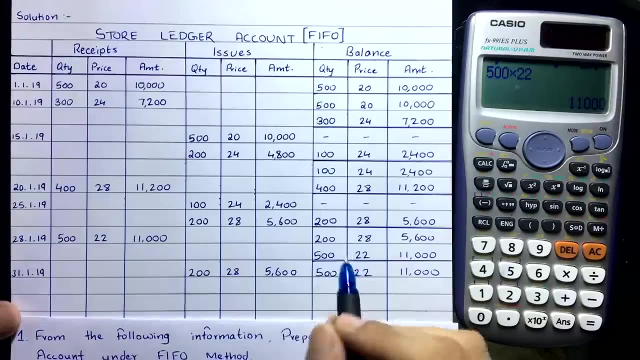 on january 31. what is happening on january 31? you have issued 200 units. you have issued 200 units. 200 units are going out of the warehouse. simple, it's not tough. see here now what you have in the warehouse. you have this lot- yeah, these two lots. you have 200 and 500 lot- yes, 200 was the previous. 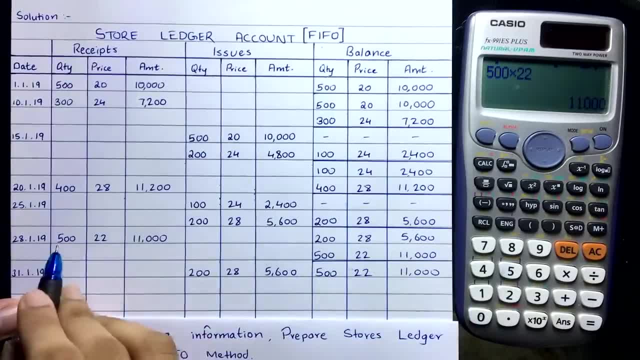 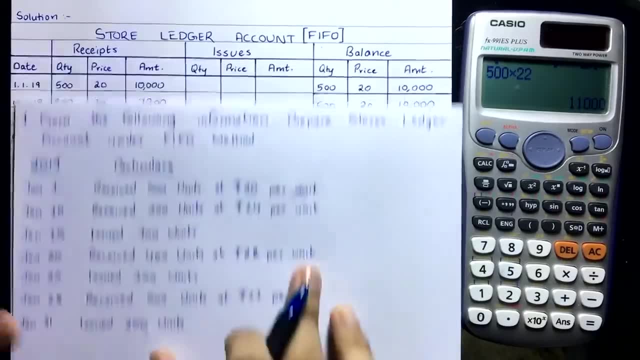 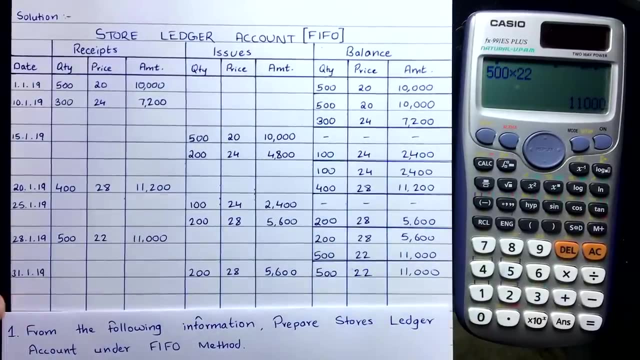 lot and the 500 was? you received it right just previously? 500, yes, okay. so now you have to send out 200, 200 units, as said in the question. 200 issued 200 units. so how will you do that? simple, this entire lot, you can send it out right. 228, 5600. so what is left? that thing is entirely gone. yeah, 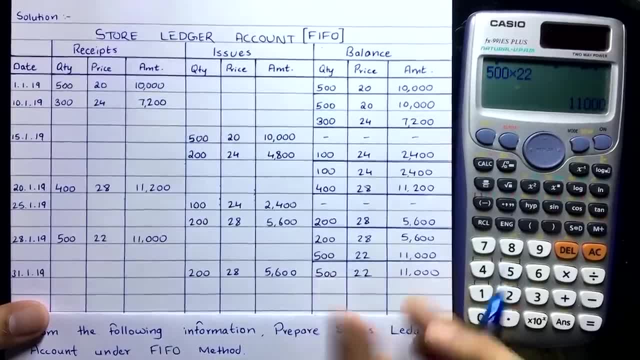 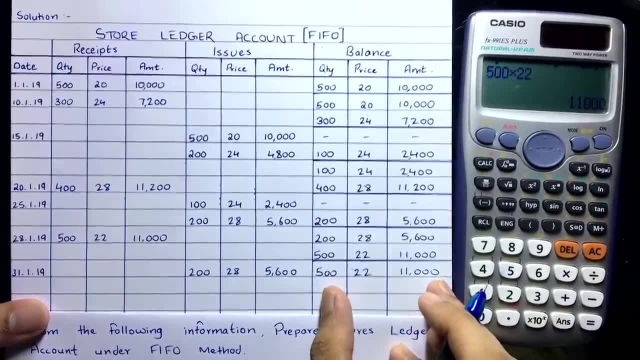 you can take it nil, nil, nil, and you can take whatever that is left below also. yeah, but i've not taken nil nil over here. it's your choice. okay, so i've directly taken 520 to 11 000. this is the closing stock now. this is what is left in the warehouse. this much. 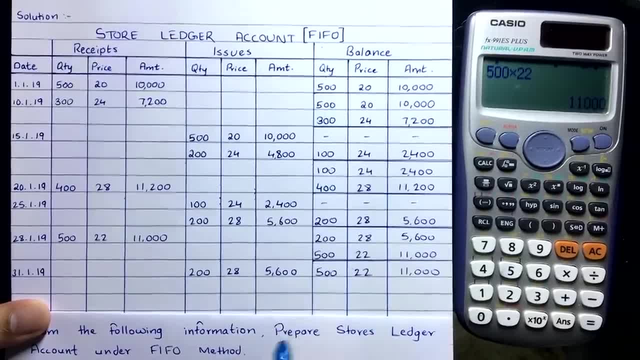 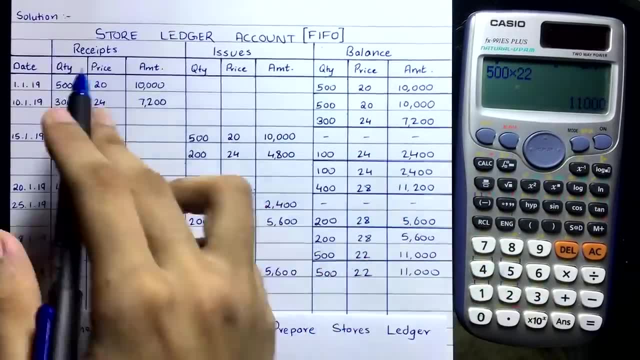 balance. yeah, so you can write that down below. also: closing stock colon 520 to 11 000. okay, simple as that. so this is how you have to do the fifo method. yeah, this is how you have to prepare the store ledger account. whatever that comes in first, you have to throw that out, you have to send it out. 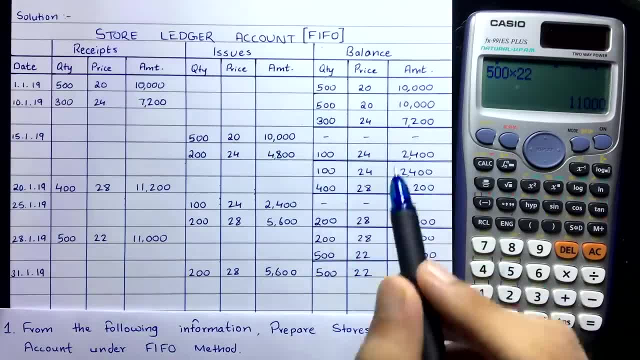 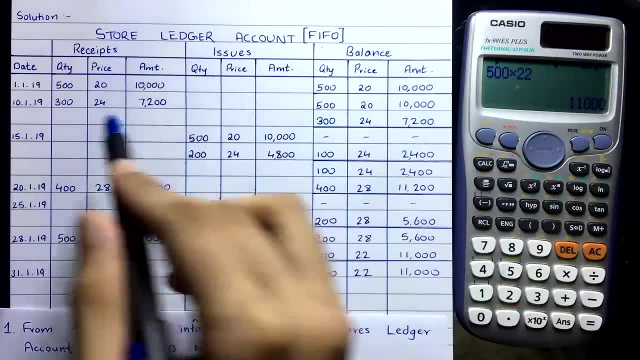 you have to be careful about is the balance column. yeah, how to do the balance column: whenever you get a receipt, you know, draw a line, copy whatever that is there in the balance column previously down, yeah, and then copy the new thing exactly down. simple, right. so now in the next video we are